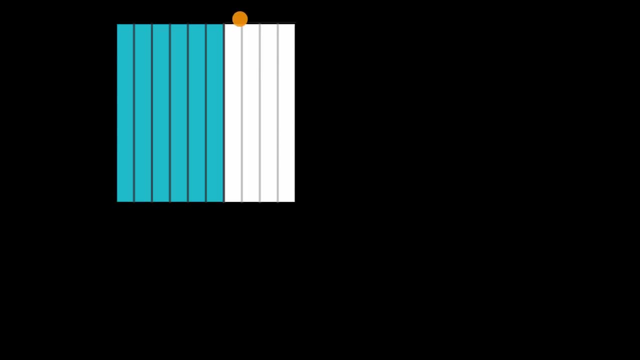 So let's assume that this entire square represents a whole And we can see that part of it is shaded in in blue. What we're going to do in this video is try to represent the part that is shaded in blue as a fraction, as a decimal. 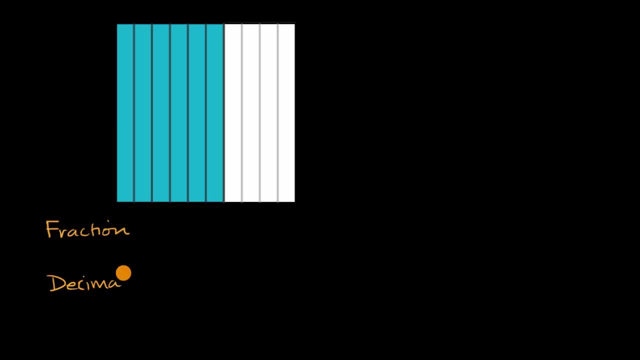 decimal, decimal and as a percent. So pause the video and see if you can do that. Well, let's first think about it as a fraction. So the whole is split into one, two, three, four, five, six, seven, eight, nine, 10 equal sections. 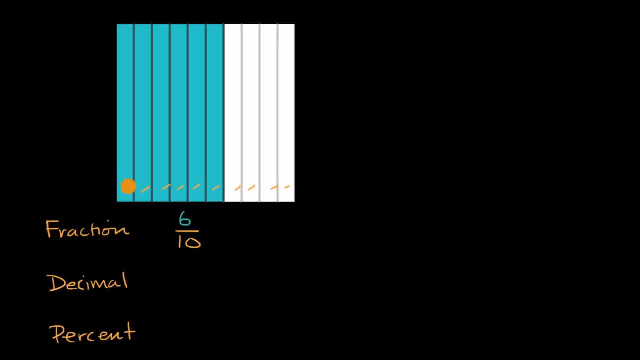 And six of them are filled in. So the blue represents six tenths of a whole, or represents, you could just say, six tenths, And you could also rewrite that If you divide the numerator and the denominator by two, that's the same thing as three over five. 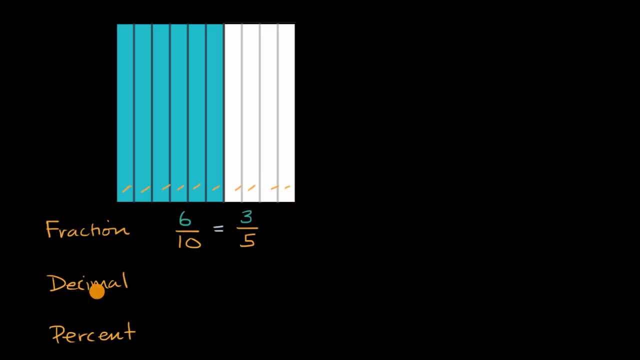 Fair enough. Now let's represent it as a decimal. What decimal would it be? Pause the video again and see if you can do that. Well, six tenths: we could literally just go to our place value. So that's the ones place we have a decimal. 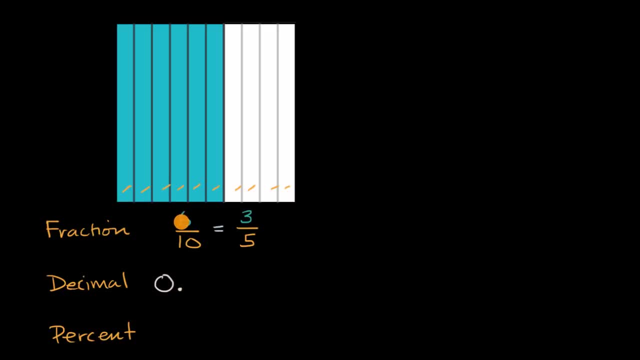 And then you have your tenths place, And so we have six tenths. so you could just put it right over there: We are putting a six in the tenths place to represent six tenths. Now, what about a percentage? Well, percent means per hundred. 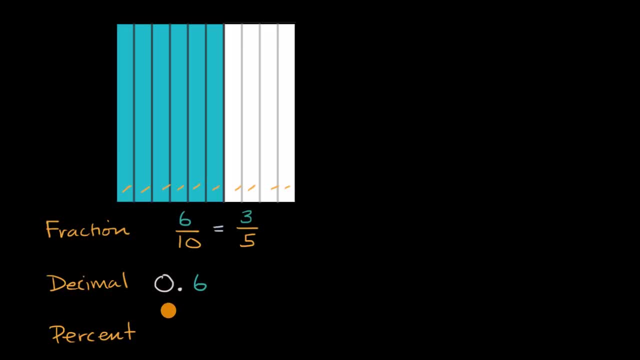 So one way to think about it is: six over 10 is the same thing as what per hundred That is equal to. if we multiply the numerator and the denominator by 10, that's the same thing as 60 per hundred, Or another way of thinking about it. 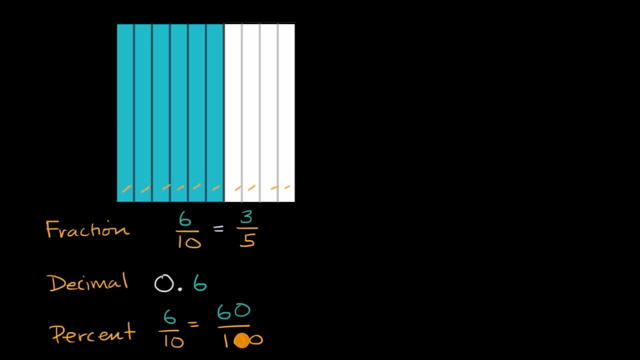 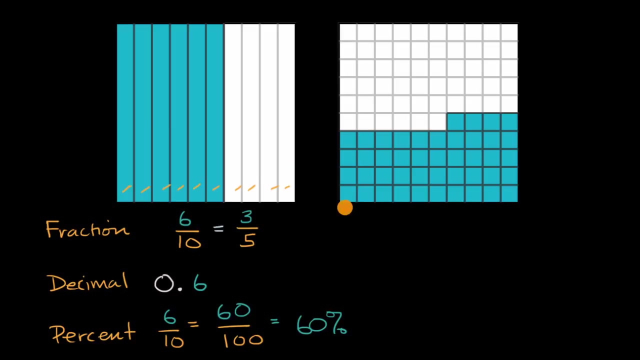 60 per. instead of hundred, you could say cent, And so this would be equal to. this would be equal to 60 per hundred. Okay, 60 percent. Let's do another example. So here, once again, our entire square represents a whole. 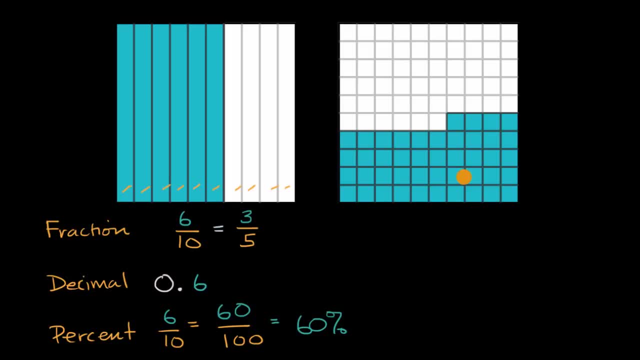 So see if you can represent this as the part that's shaded in blue as a fraction, Pause the video and do that. Well, you can see that this is a 10 by 10 grid, So there's a hundred equal sections here. 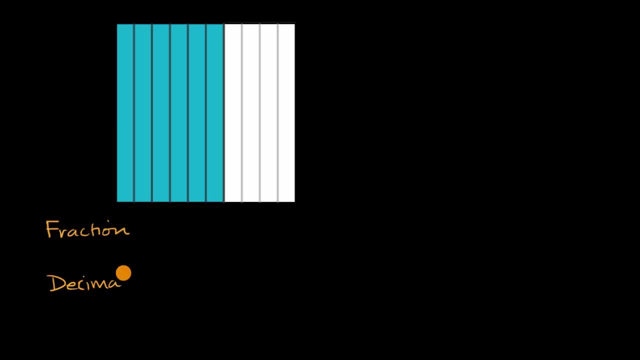 decimal, decimal and as a percent. So pause the video and see if you can do that. Well, let's first think about it as a fraction. So the whole is split into one, two, three, four, five, six, seven, eight, nine, 10 equal sections. 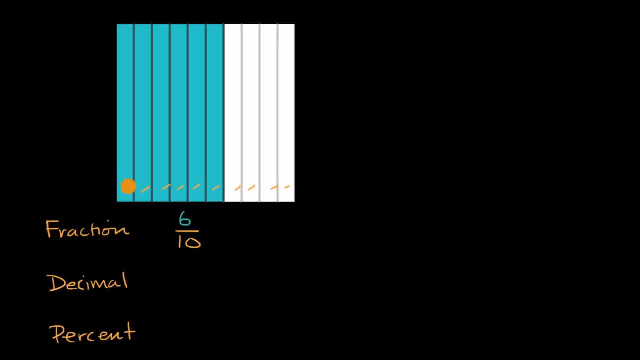 And six of them are filled in. So the blue represents six tenths of a whole, or represents, you could just say, six tenths, And you could also rewrite that If you divide the numerator and the denominator by two, that's the same thing as three over five. 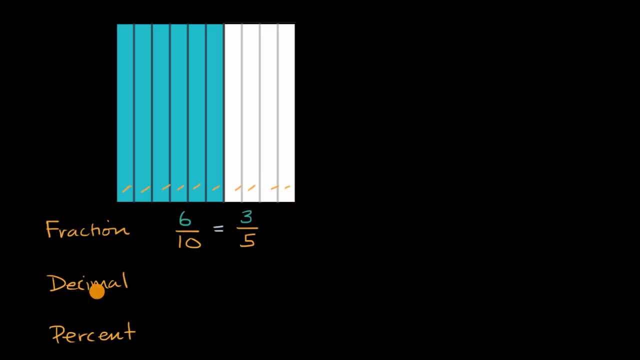 Fair enough. Now let's represent it as a decimal. What decimal would it be? Pause the video again and see if you can do that. Well, six tenths: we could literally just go to our place value. So that's the ones place we have a decimal. 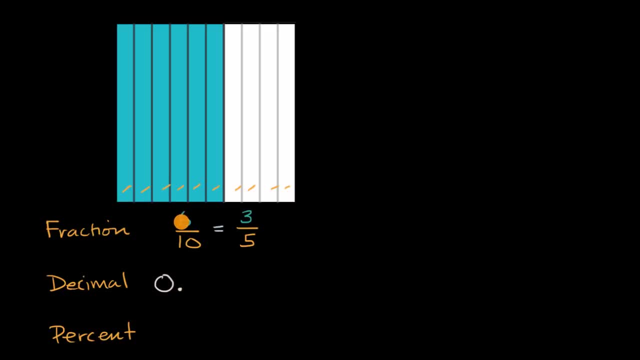 And then you have your tenths place, And so we have six tenths. so you could just put it right over there: We are putting a six in the tenths place to represent six tenths. Now, what about a percentage? Well, percent means per hundred. 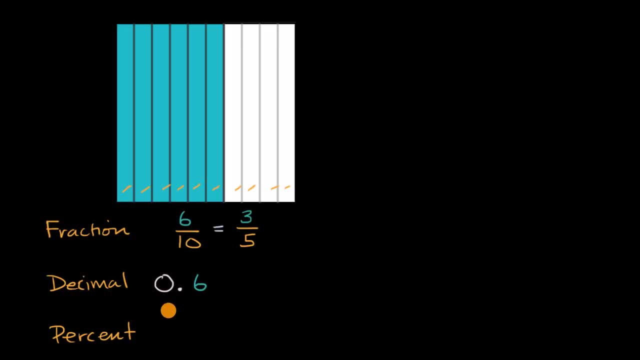 So one way to think about it is: six over 10 is the same thing as what per hundred That is equal to. if we multiply the numerator and the denominator by 10, that's the same thing as 60 per hundred, Or another way of thinking about it. 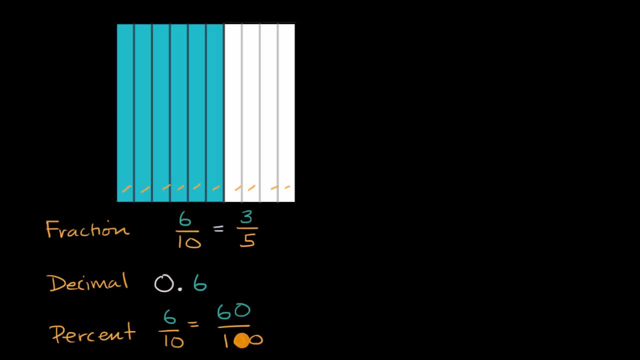 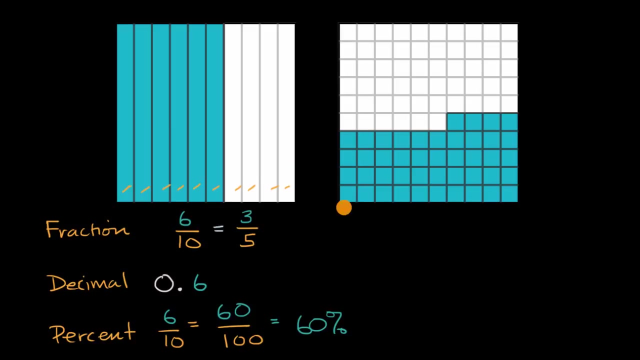 60 per. instead of hundred, you could say cent, And so this would be equal to. this would be equal to 60 per hundred. Okay, 60 percent. Let's do another example. So here, once again, our entire square represents a whole. 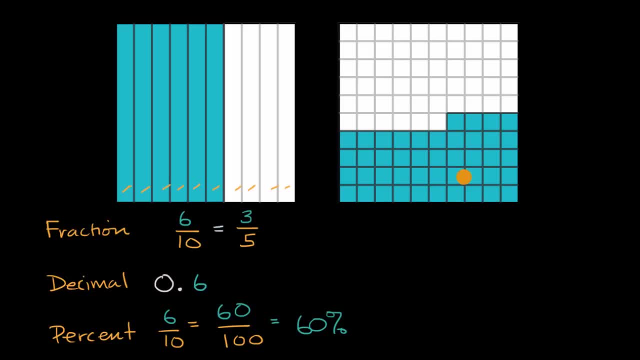 So see if you can represent this as the part that's shaded in blue as a fraction, Pause the video and do that. Well, you can see that this is a 10 by 10 grid, So there's a hundred equal sections here. 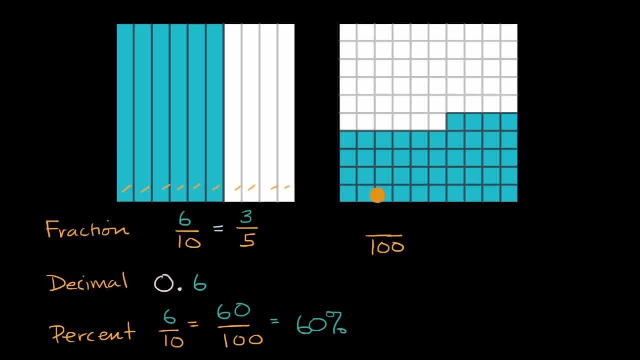 A hundred equal sections. Each of these squares represents one hundredth, And how many of them are there? This is this row is 10, 20,, 30,, 40, and then one, two, three, four. So this is 44 over a hundred.